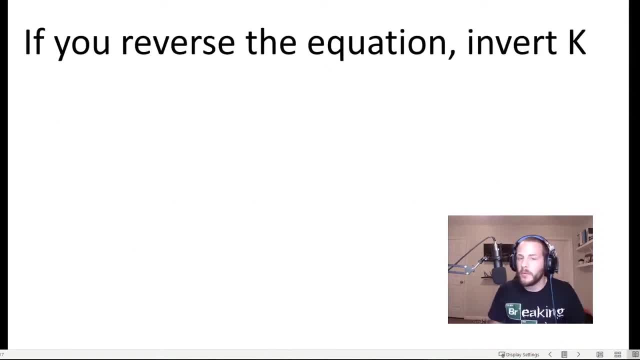 looked at in that little bulleted list was if you reverse a chemical equation. So if you reverse a chemical equation, what does that do to the equilibrium constant? Well, it inverts it, right. If you reverse the chemical equation, you invert the equilibrium constant, right. So 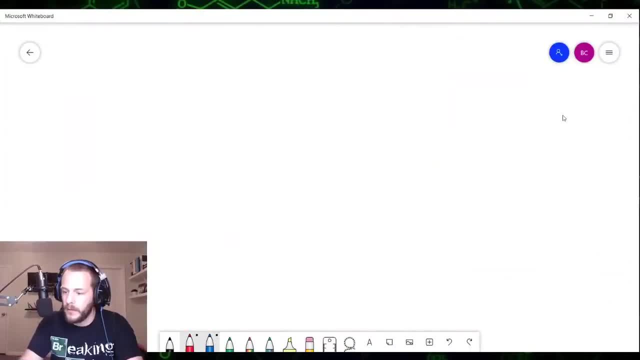 to demonstrate this, I'm going to go to the whiteboard. Let's say we have a chemical equation that looks like this, where we have A plus 2B reacting at equilibrium to form 3C, right? So this is just a general equation. right Now we know from the law of mass action that this reaction 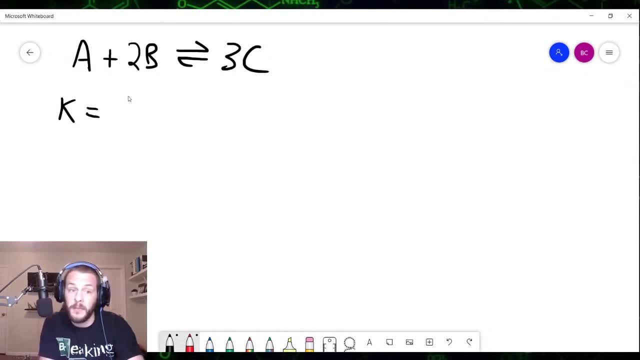 or, excuse me, that the equilibrium constant associated with this reaction is going to be the: the concentration of C to the third power cubed times the concentration of A, or, excuse me, divided by the concentration of A times the concentration of B squared. So we know that. 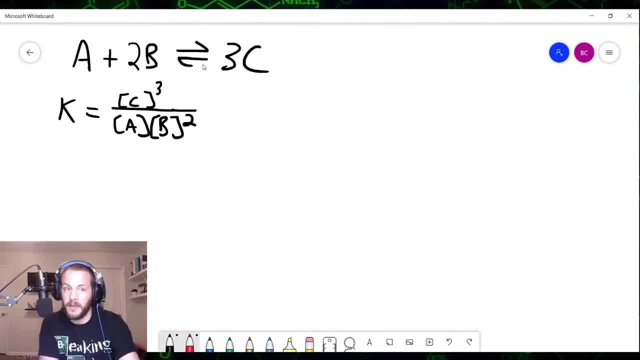 this is the expression for the equilibrium constant for a reaction that looks like this right Now: if we had the reverse reaction- so I'll do that in blue. So let's say we had the reverse reaction- products become reactants, reactants become products- We would have 3C. 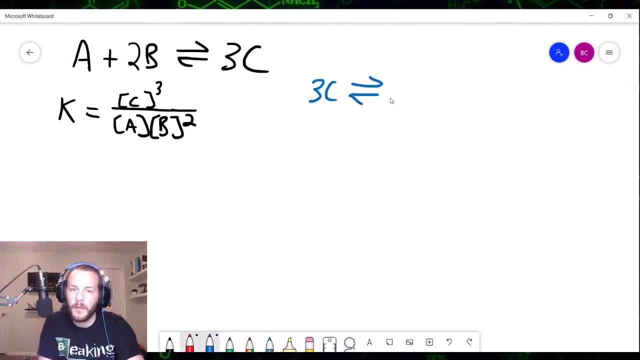 reacting to form, to form A plus 2B. right, And so this reaction, I'll call it K minus 1, the reverse rate constant or not rate constant C- Here I just got it mixed up too. The reverse equilibrium constant. 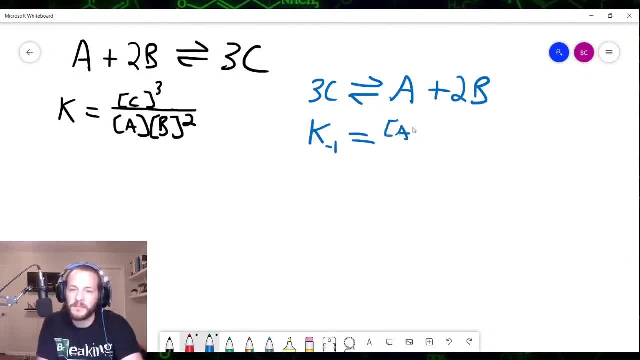 would be concentration of A times concentration of B, squared divided by the concentration of C, cubed right, And so we can see here that the expressions for the equilibrium constant between the forward reaction and the reverse reaction are flipped. All we've done is we've just taken the reciprocal 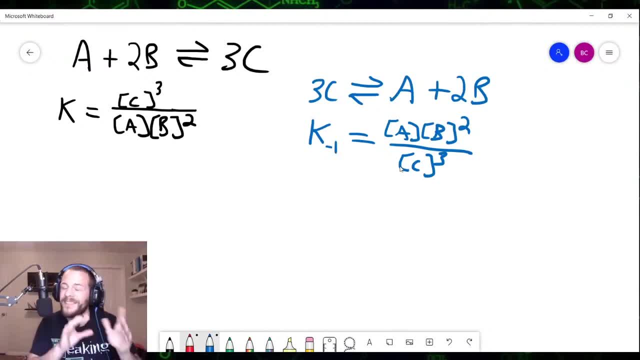 the inversion of one rate or one equilibrium constant to arrive at the other. And so we have this relationship here where the K minus 1 is simply equal to 1 over K, right? So if you have an equilibrium constant and you want to know the equilibrium constant for the reverse reaction, 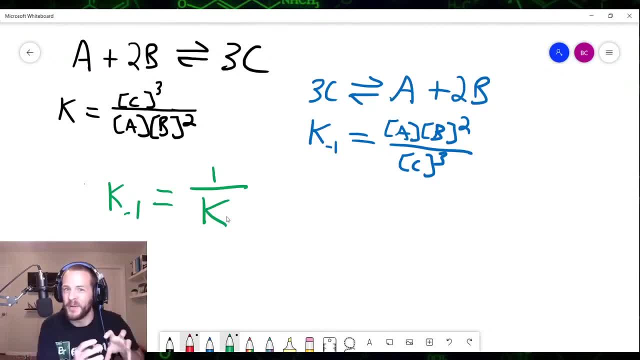 all you've got to do is take one and divide it by that original equilibrium constant and voila, there you are. There's the equilibrium constant for the reverse reaction. So I hope everybody's following, because we are going to move on with the second scenario. 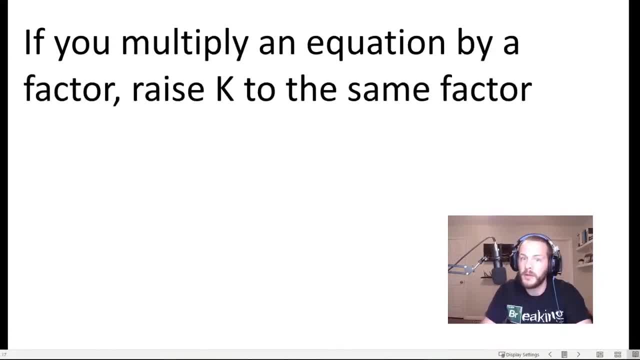 So the second scenario is that if you multiply an equation by a factor- so in other words, if I take all the coefficients of a balanced chemical equation at equilibrium and I multiply that by some factor, what you're going to do is you're going to raise the equilibrium. 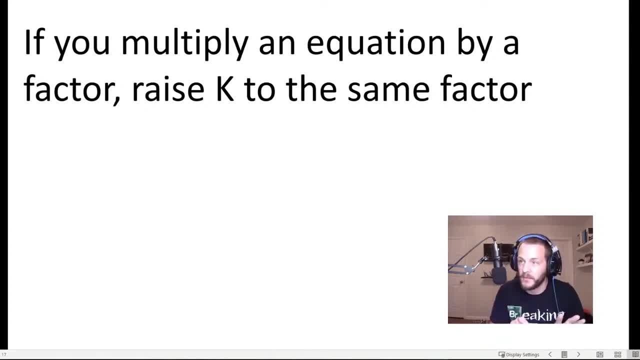 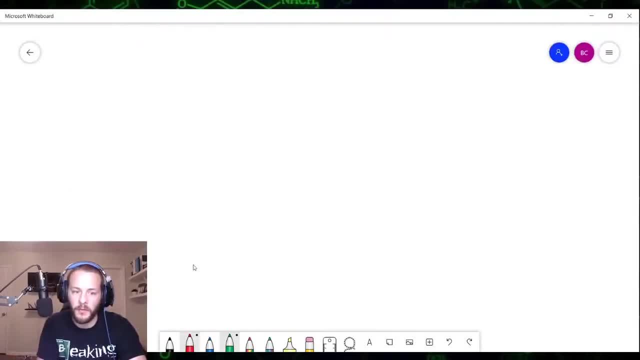 constant to the power of that same factor. So, just like in the previous example, I'm going to show you again how the mathematics works behind this. If we go back to that same scenario- I wish I didn't erase it a moment ago, because I'm using it again. so if we go, 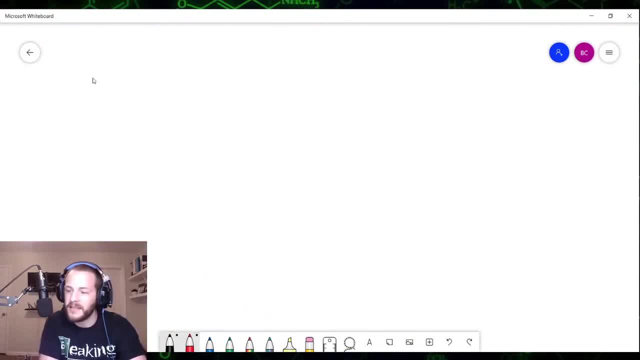 back to that same scenario right where we have, let's see A plus 2B reacting to form C right, And of course the equilibrium constant for this is K is equal to concentration of wait. I said 3C. that's what it should be: 3C right. Concentration of C cubed divided by concentration. 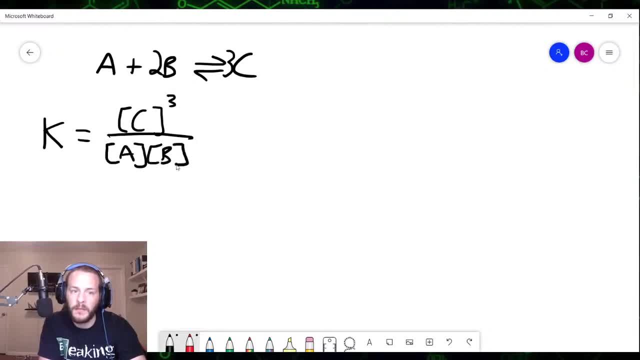 of A times concentration of B, squared right. So that's the equilibrium constant for the original reaction. right Now, imagine that I multiply this equation by some factor which we will call N, right. So the resulting equation would be N times A plus 2N times B, reacts to form 3N times C. So again, if you multiply, 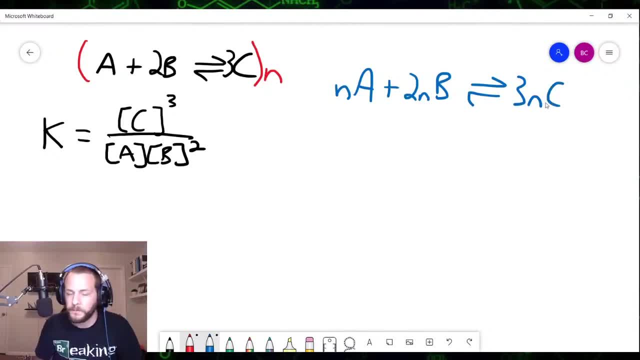 an equation by a factor, you're multiplying all of the coefficients in that equation by the same factor, right Okay? so how does that affect the equilibrium constant? Well again, if we apply the Law of Mass Action once again, we get that K, Father and I'll. 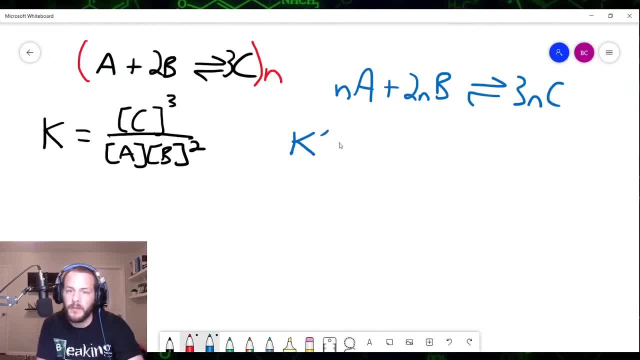 just call it K-prime. K-prime is equal to concentration of C to the 3N right, raised to its coefficient, divided by the concentration of A to the N times, the concentration of 2B cubed of B, two cubed. 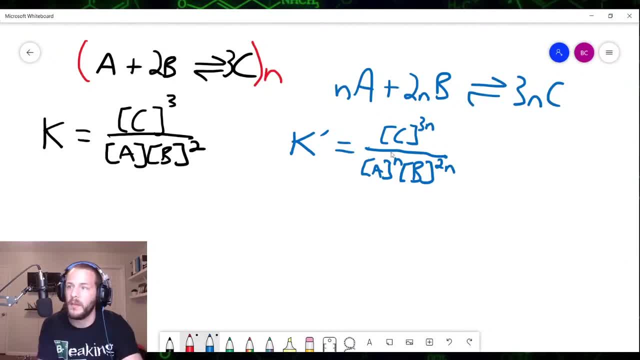 ofN squared to the 2n right. This expression here simplifies down, just because of the properties of exponents to the concentration of C cubed divided by concentration of A times concentration of B, squared this whole thing to the power of n right, And so we arrive at the relationship. 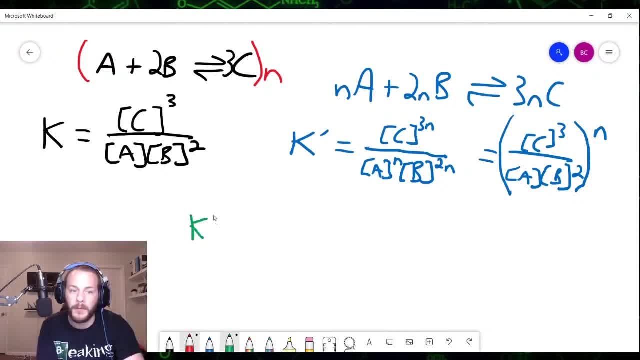 that we talked about before, where we have k, prime is equal to the original equilibrium constant, k to the power of n, Whichever factor it was that you multiplied by the original equation. you take the equilibrium constant, you raise it to that factor and that gives you. 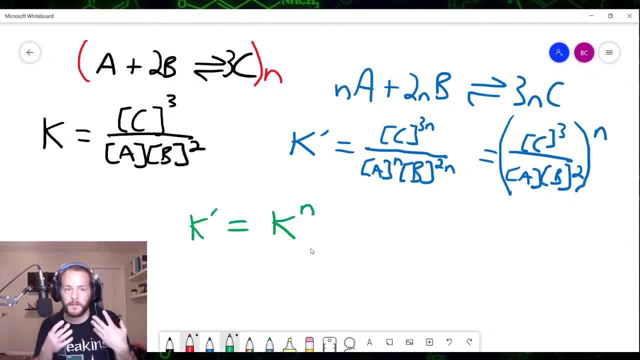 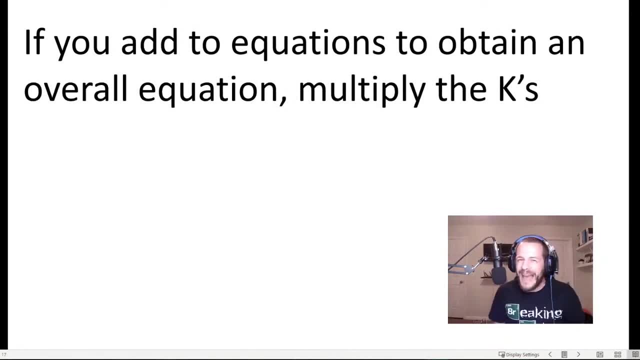 the equilibrium constant associated with your new equation. Alright, So the third possibility, the third type of manipulation that you might be asked to perform on a chemical equation and understand what to do with its equilibrium constant, has to do with adding equations together. So if you add equations together to obtain an overall balanced chemical equation, 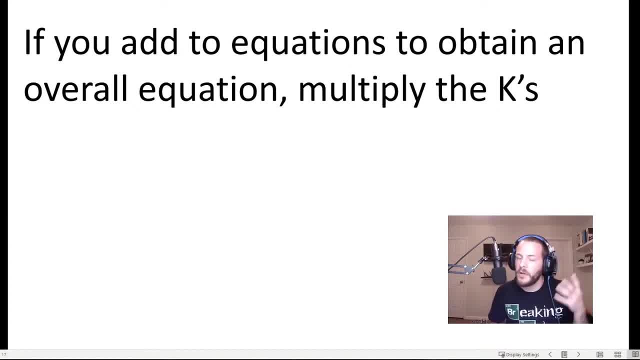 what do you do? Well, you're going to multiply the equilibrium constant. You're going to multiply the equilibrium constant constants for those individual summed reactions to arrive at the equilibrium constant for your summation, for your overall reaction. and so I can, once again, 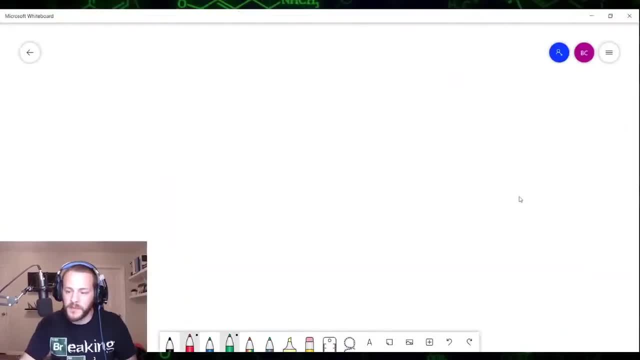 go to the whiteboard and explain how this works from a mathematical point of view. so let's say that you have two reactions that you're adding together. the first reaction let's say that it is a reacting to form 2b. and then let's say: 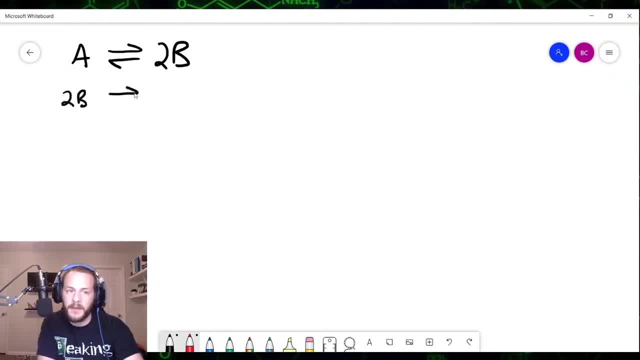 that you have to be reacting to form 3c, right? so those are your two equations that you add together, and then your your two B's would cancel. once you add those together and the overall equation that you would get would be: a is reacting to form 3C, right? so what would the equilibrium constants look like for? 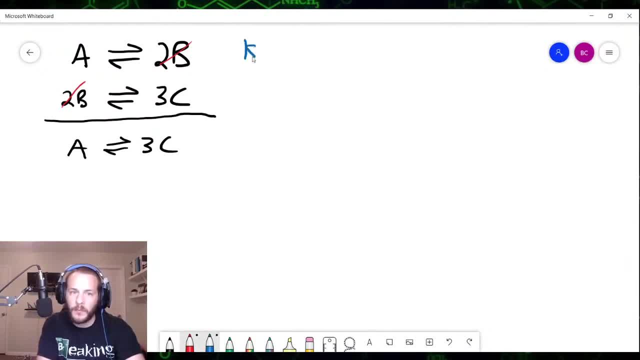 these reactions? well, this one, I'll call it k1, is equal to what is it going to be? what do you think it's going to be? it's going to be concentration of B squared over concentration of A. and then this one down here, k2. I'll call it k2, not to 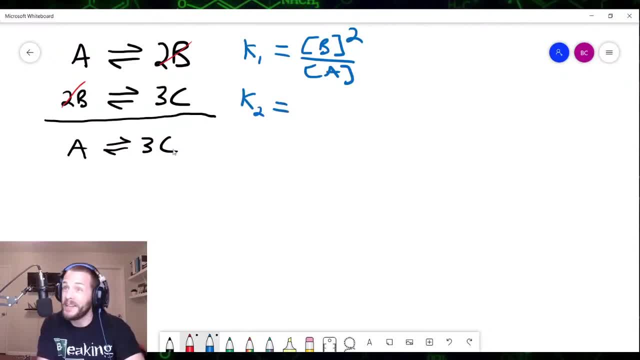 be confused with something that you should never ingest. the second equilibrium constant is going to be concentration of C cubed divided by concentration of B squared right, and this one down here, which I'll call k O just for overall, is going to be concentration of C cubed divided by: 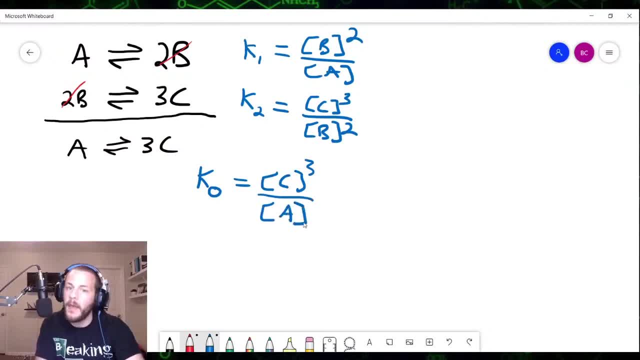 concentration of A right. so notice that if we take k1 and multiply it by k2- and I'm going to try to do this little fancy lasso thing here- I'm going to lasso this k2 expression right here and I'm going to bring it over there. so imagine I'm multiplying. 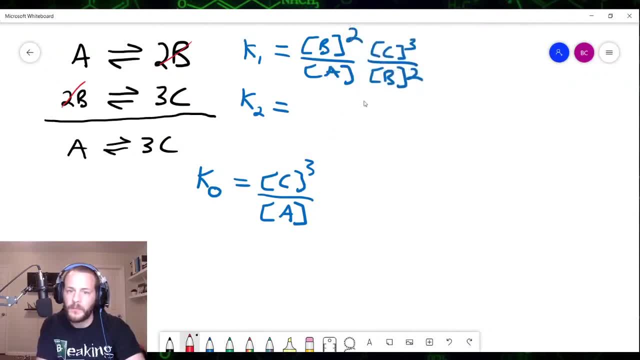 these together. right. then you see, my concentration of B squared terms are going to cancel and I'll be left with concentration of C cubed over concentration of A. so it makes sense, right. there's a reason why multiplying the equilibrium constants for the individual reactions arrives at the 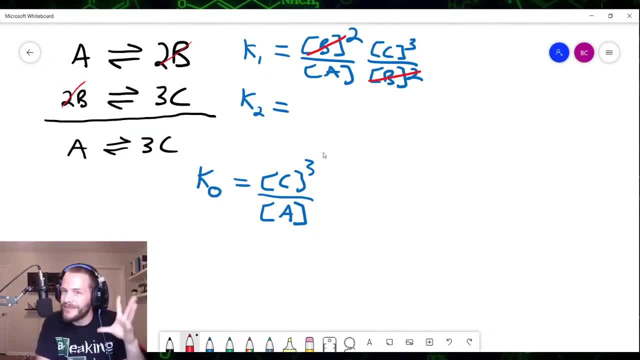 equilibrium constant for the overall. so I could have just told you guys that that's how it works, right. I could have just told you the rules, but I always like to make sure I'm explaining things and make sure people kind of get an understanding mathematically of how this works. I don't like to just spoon feed. 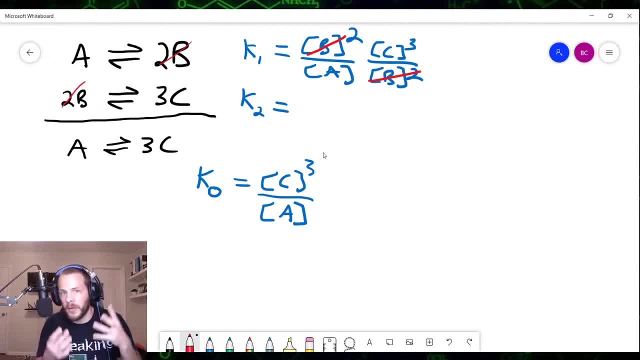 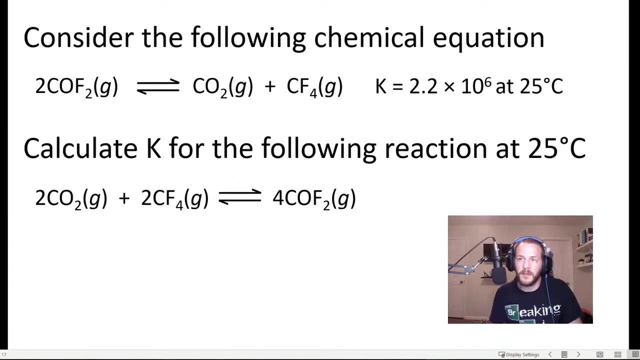 you a formula and expect you to follow it. I really, really want you to understand the mathematics behind it. So I really hope you've appreciated that and you've found value in it. So let's do a problem where we put that knowledge to work. So it says to consider. 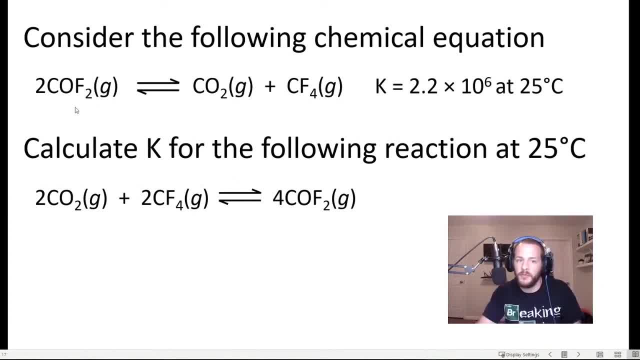 the following reaction where we have 2COF2 reacting to form CO2 and CF4, and that has an equilibrium constant of 2.2 times 10 to the 6th at 25 degrees Celsius. Now the at 25 degrees. 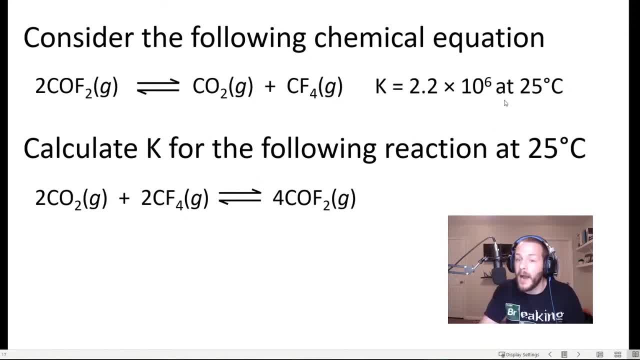 Celsius part might seem insignificant, but it's not. Equilibrium constants do depend on temperature and we will certainly talk about that in a later live stream. but just understand for now that equilibrium constants do change with temperature. So the problem asks us to calculate the equilibrium. 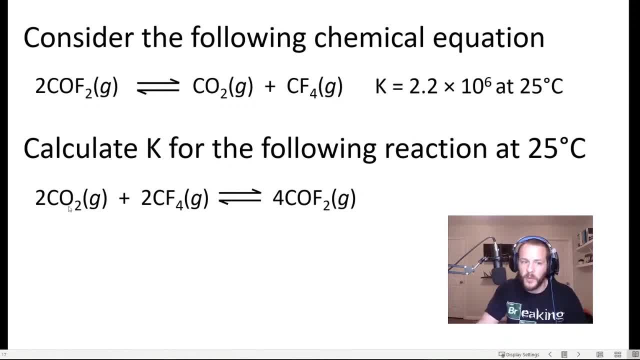 constant for this reaction. So we have 2CO2 plus 2CF4 reacting to form 4COF2.. So the main idea here is that this equation, for which we're trying to find the equilibrium constant, is the result of one or more manipulations. 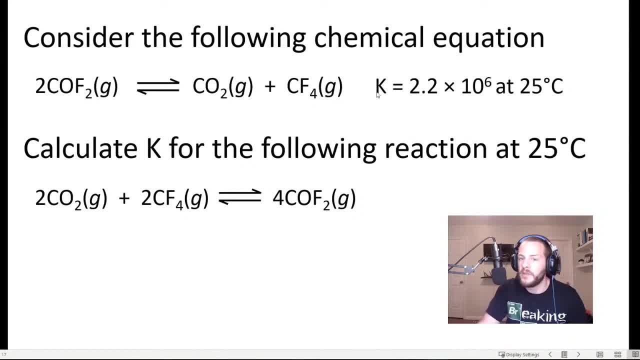 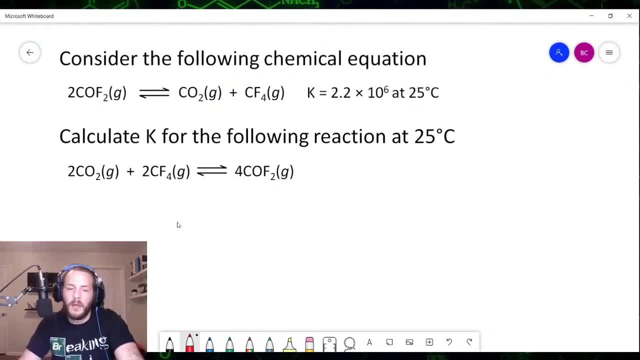 to this equation up here, in which the equilibrium constant is already given. So we need to come up with a plan for how we're going to manipulate this equation To get from the reaction that we started with to the reaction that we end up with, and we 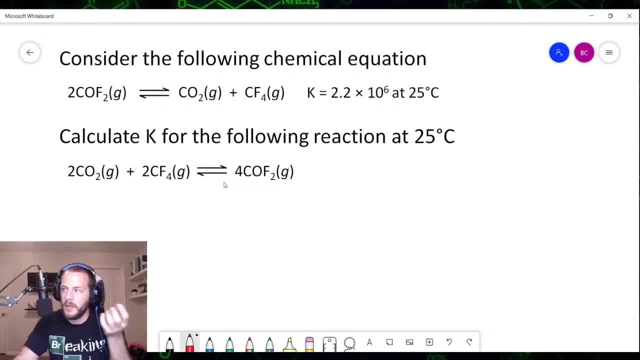 need to make sure that we understand those relationships involving the equilibrium constant. along the way. I don't know about you, but this kind of reminds me of those delta H- Hess's law problems where you manipulate delta H based on manipulating chemical equations. That's the impression that I got when I first started studying this Type a message in the. 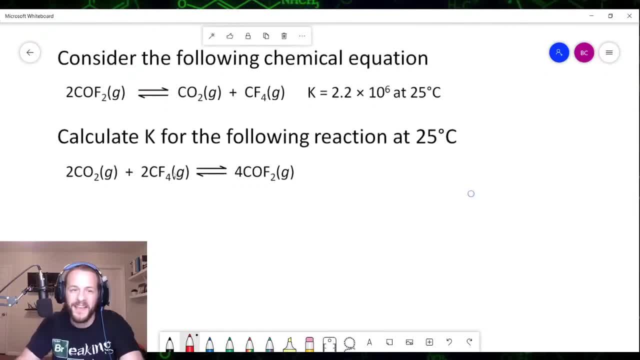 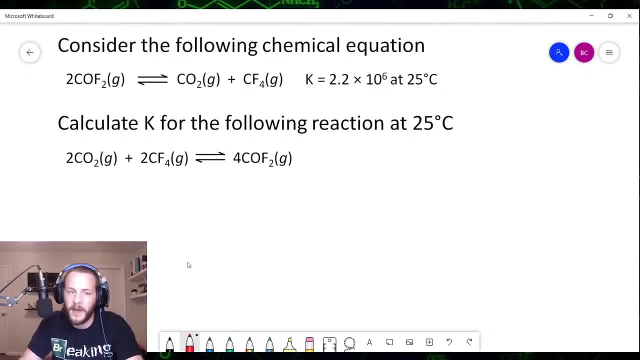 chat if you feel the same way or not. Whatever you want, All right. So We can see. we can clearly see, right, that we're going to have to reverse this chemical equation right, Because in the example that we're given, we have COF2 on the left and 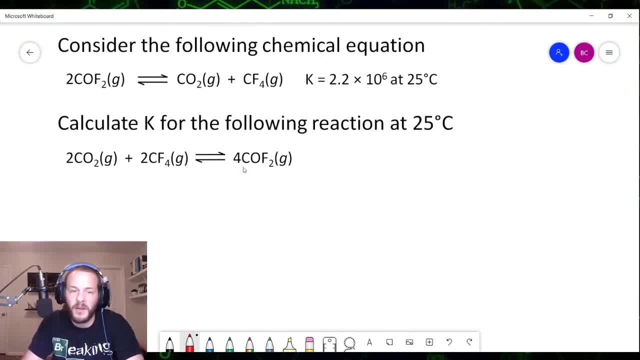 in the example, in the target equation. I'll just call this the target equation. from here on out, we have the COF2 on the right, So we definitely have to reverse this equation. That's not all that we have to do, but that's at least one thing that we have to do. So 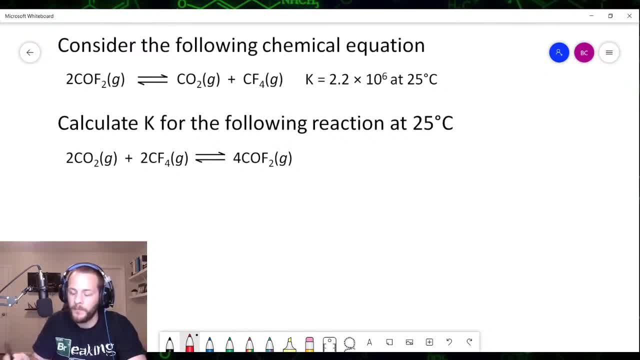 why don't we start with that right? So if we take this equation up here, right, and we reverse it, well, what are we going to end up with? Well, that equation is going to be: CO2 plus CF4 yields 2COF2.. 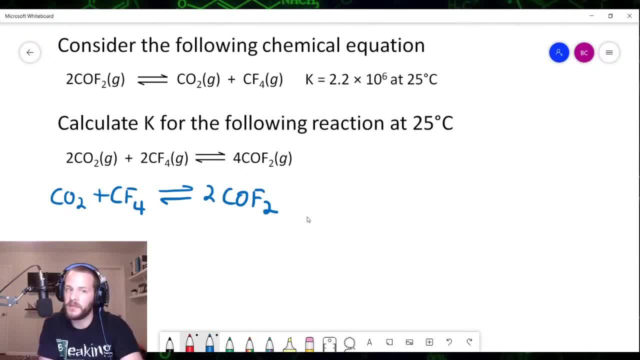 If we recall from those rules that we discussed earlier, when we reverse a chemical equation, we invert COF2.. We take 1 over the equilibrium constant right, And so for this reaction, K is going to be 1 over this original equilibrium constant, 2.2 times 10 to the sixth right, 1 over 2.2. 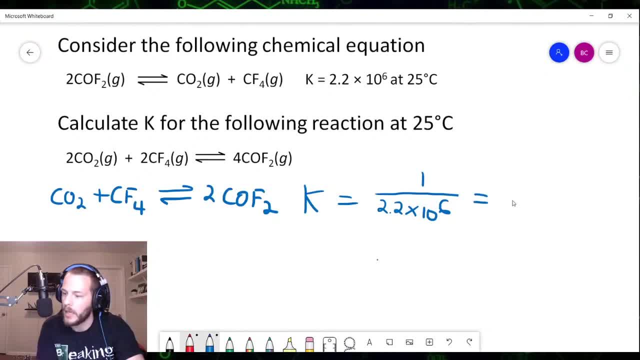 times 10 to the sixth. So I got 4.5 times 10 to the minus 2.. I got 4.5 times 10 to the minus 7, right, So this is our equilibrium, constant upon reversing the equation that we started with. 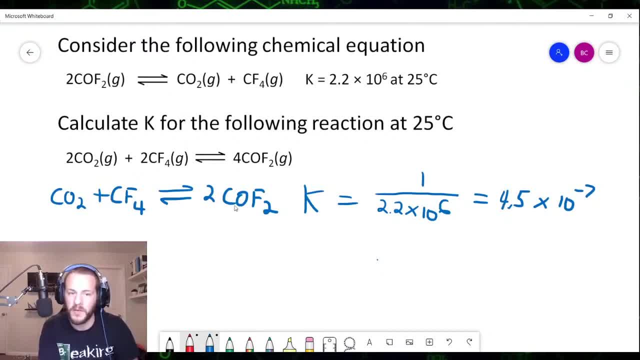 Now we still have to do more work, right, because this equation is not identical to the target equation. To get our target equation, we have to multiply this equation by a factor. We have to multiply this by a factor of looks like. looks like it's going to be 2, right. 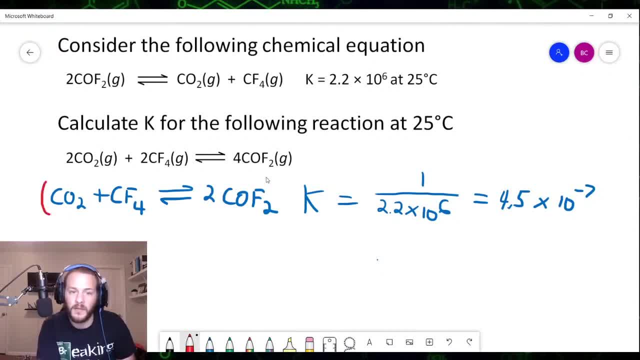 So we need to take this equation And we need to multiply that by a factor of 2, right? And so, in doing that, what we're going to end up with is an equation that looks like this: It's going to be our target equation, right? 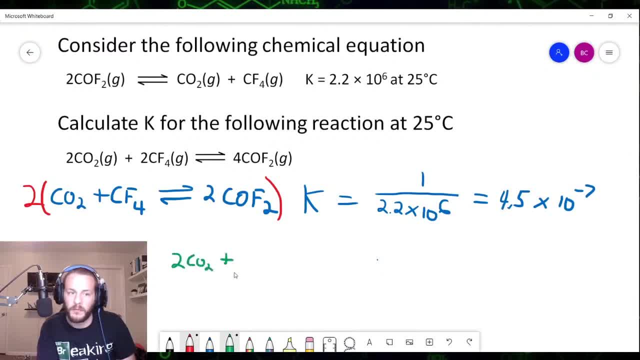 2CO2 plus, excuse me, yeah, 2CO2 plus 2CF4 yields 4COF2.. Right Right, Right, Right 2.. So that's our target equation. That's what we want. 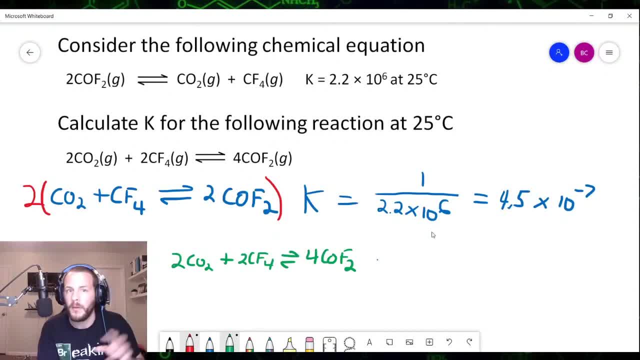 And remember from the rules that we talked about earlier, when we multiply an equation by a factor, we're going to raise the equilibrium constant to the power of that factor, So this equilibrium constant that we just calculated here. what we're going to do is: 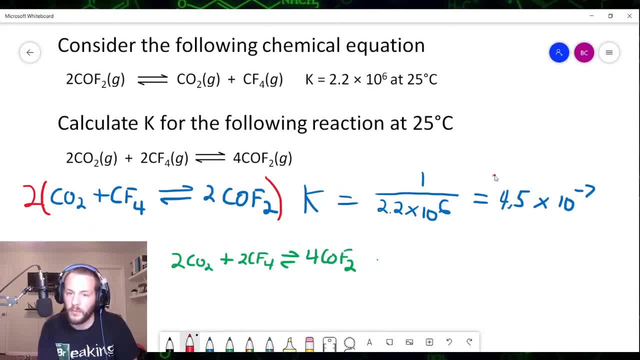 we're going to take that and we're going to square it, We're going to raise that to the second power And the number that you end up with. and again, I would highly encourage anybody who has a calculator, who might be watching, to perform this calculation for yourself. just.